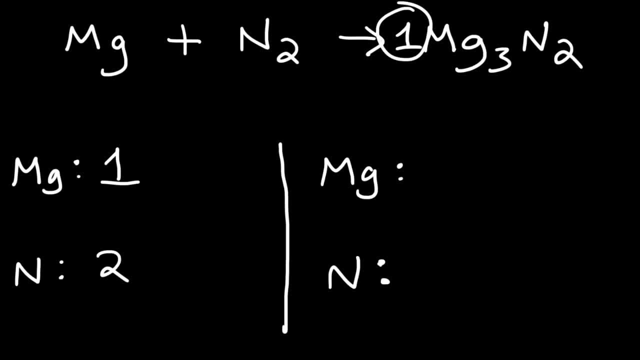 So 1 times 3 is 3, which means that we have three magnesium atoms and only two nitrogen atoms. 1 times 2 is 2.. So right now, looking at the left side and the right side, we can see that the number of nitrogen atoms are the same. So we don't. 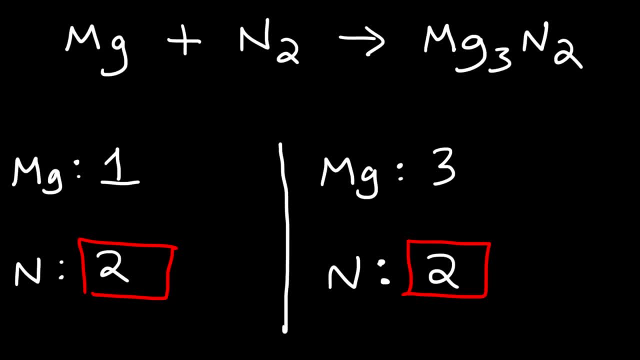 have to worry about that. However, the number of magnesium atoms: they're different, So what do we need to do to make them equal? What we need to do is multiply this number by 3.. And we can do that by putting a coefficient of 3 in front of mg. Now it's important to 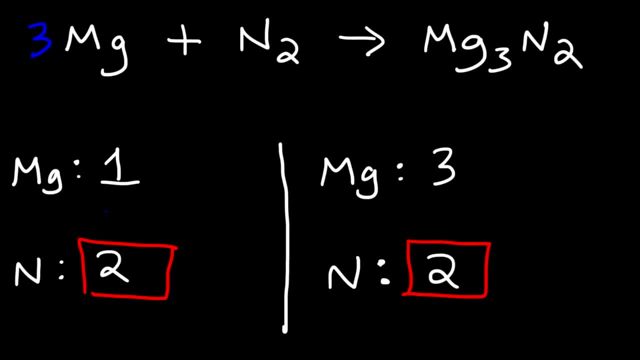 understand that when balancing equations you could change the coefficient but you cannot change the subscript. Make sure you understand that. So you cannot change this number Now. once we put a 3 in front of mg, this number changes. So now we have three. 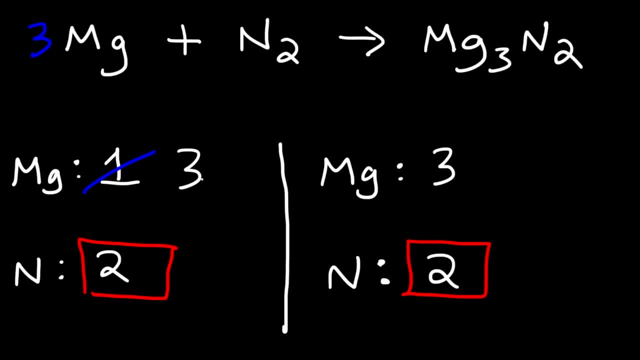 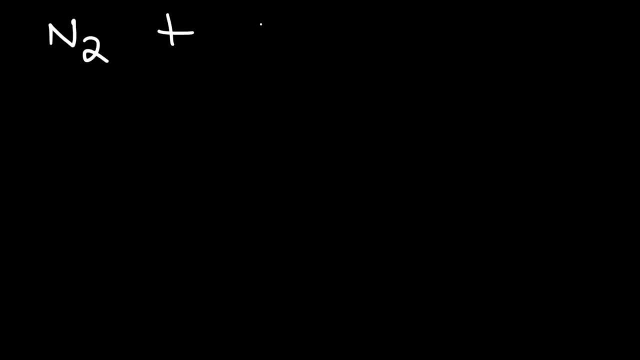 magnesium atoms on both sides of the equation. So at this point the equation is balanced. Now let's work on another example. Let's react nitrogen gas with hydrogen gas to make ammonia, NH3.. So, using the same techniques as the last, 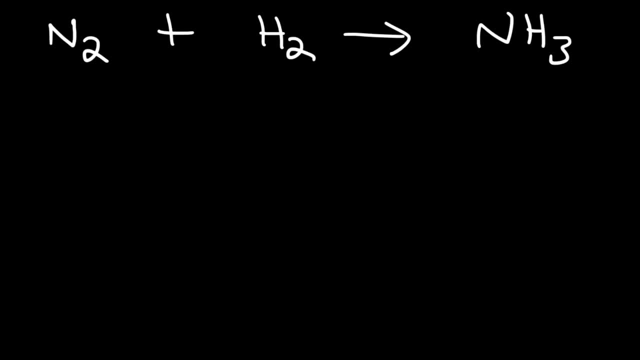 example. go ahead and pause the video. Take a minute to work out this example. So let's make a list of the atoms that we have on the left side and on the right side. So on the left side we could see that we have two nitrogen atoms. 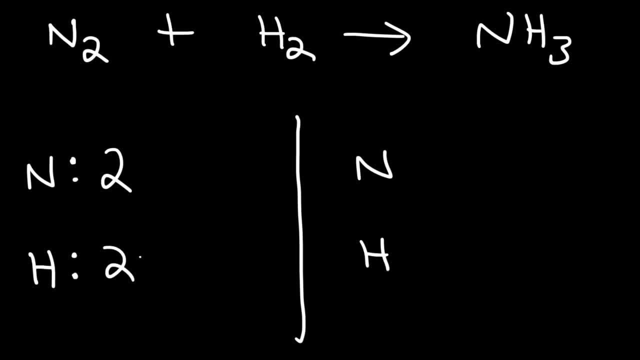 We also have two hydrogen atoms. On the right side of the equation, the product side, we only have one nitrogen atom, but we have three hydrogen atoms. So what do we need to do to make the atoms equal on both sides of the equation? Well, for one thing, we can. 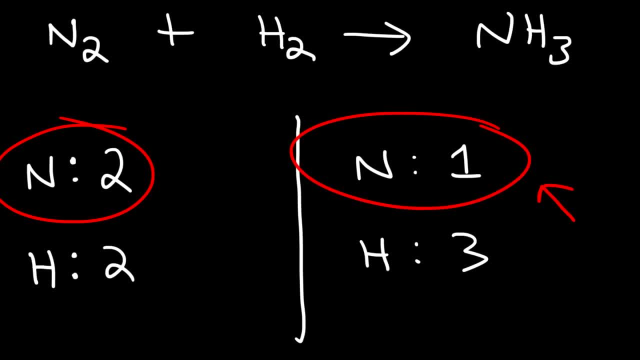 balance the nitrogen atoms by multiplying this number by 2.. So let's put a 2 on the front of NH3.. So now we have two nitrogen atoms. 2 times 1 gives you 2.. Now how many hydrogen atoms do we have on the right side? Well, if we multiply 2 by 3, that will give. 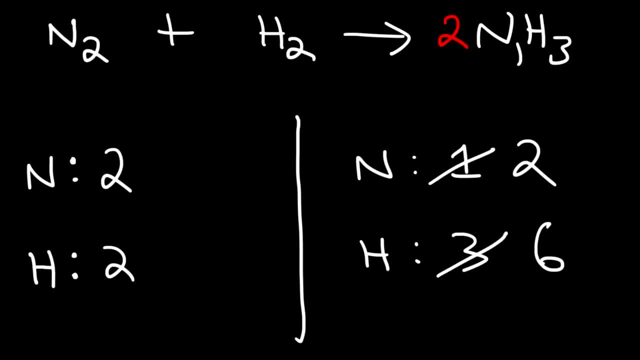 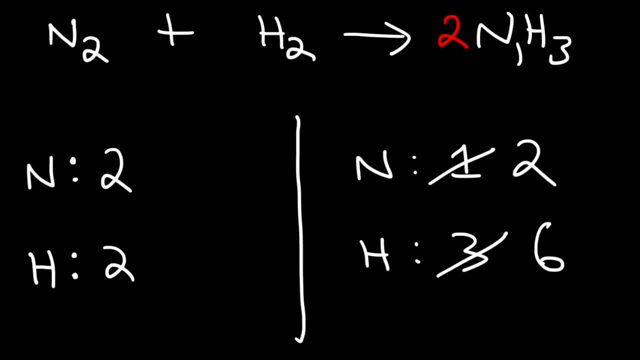 we need to multiply 2 by 3, because 6 divided by 2 is 3.. So let's put a 3 in front of N2.. I mean not in front of N2, but in front of H2, rather. 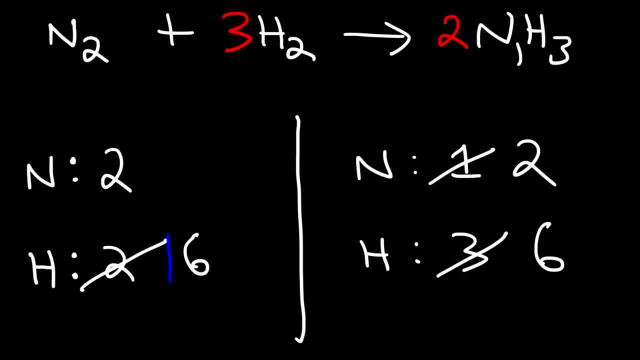 So now we have 6 hydrogen atoms on both sides of the equation And at the same time, we have 2 nitrogen atoms on both sides. So now the equation is balanced. Now for those of you who want more practice problems on balancing chemical equations: 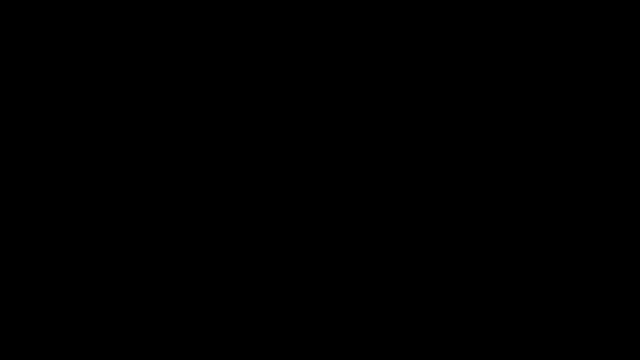 check out the links in the description section of this video. What I'm going to do is I'm going to post a few links where you can find more practice problems on balancing chemical equations, including harder examples for those of you who are looking for those challenging problems. 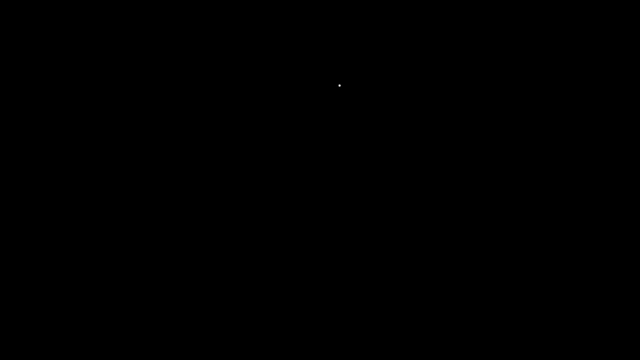 So take a look at that when you get a chance. Now let's work on the next example. So let's react elemental sulfur, which exists in the form of S8. And we're going to react it with fluorine gas to make sulfur hexafluoride. 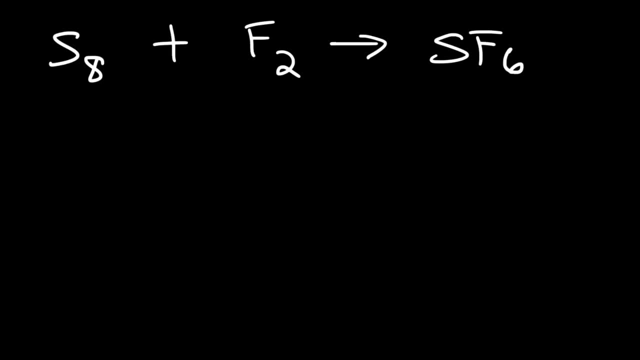 Go ahead and balance this equation. So there's two elements we need to worry about: sulfur and fluorine. On the left side we can clearly see that we have N2.. So we have 8 sulfur atoms and we only have 2 fluorine atoms. 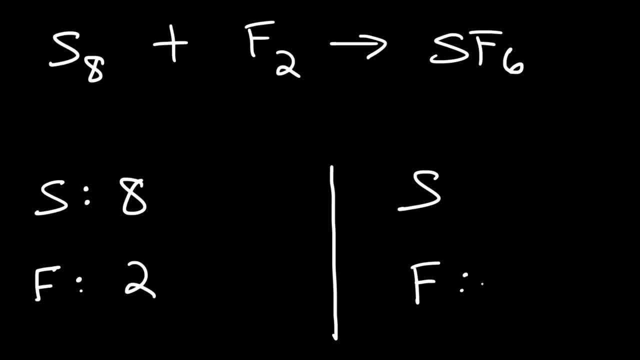 On the right side we have 6 fluorine atoms and only 1 sulfur atom. So what do you think we need to do here? Should we balance the sulfur atoms first or the fluorine atoms? Well, if we balance the fluorine atoms first, let's see what's going to happen. 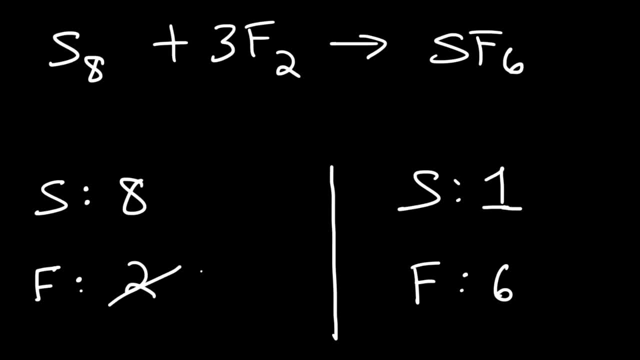 So we need to multiply fluorine by 3, because 2 times 3 will give us 6. And you can see that 3 times 2 is 6.. Next, we'll have to balance the sulfur atoms. The only way to do that is to multiply this number by 8.. 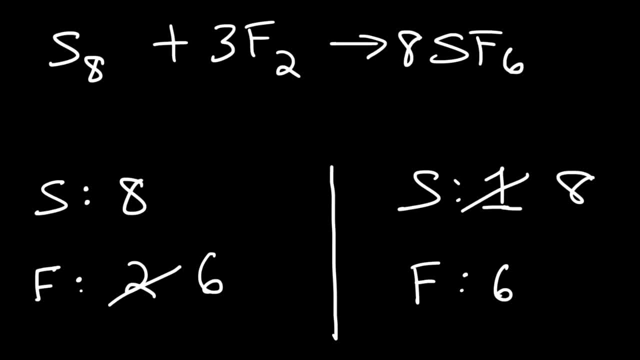 So if we put an 8 here, this will change. However, the number of fluorine atoms will change. On the right side, it's going to be 8 times 6., Which is 48. Which means that we're going to have to change this number again. 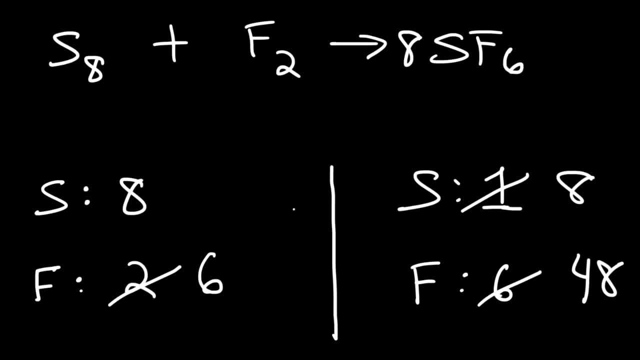 So let's go ahead and do that To get 48, if we take 48 and divide it by 2, that will give us 24.. So we need to put a 24 in front of fluorine, Because 24 times 2 is 48.. 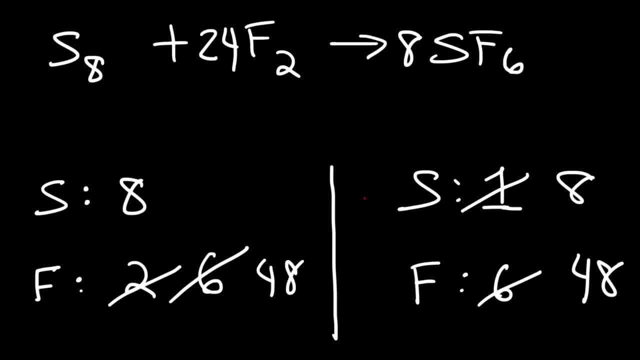 So if we multiply this number by 2, it will give us 44. So if we multiply this number by 2, it will give us 44. So now we have the same number of fluorine atoms and we have the same number of sulfur. 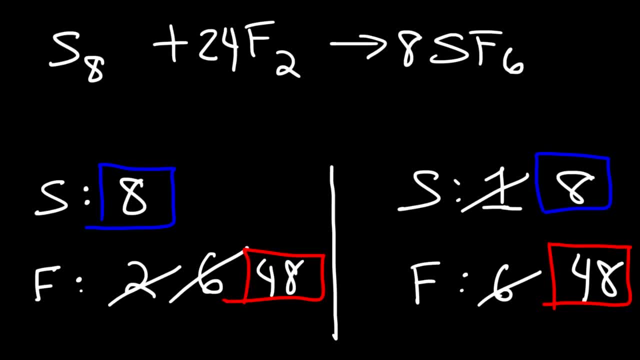 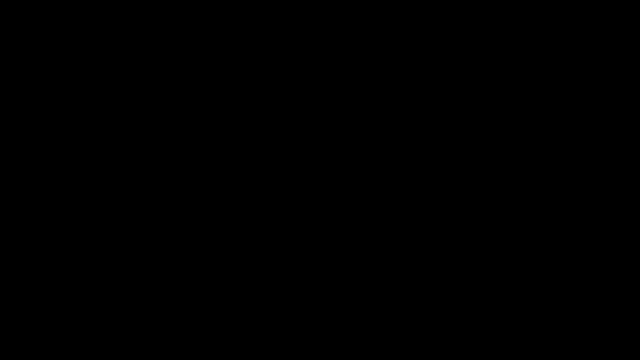 atoms. So it really doesn't matter which element you balance first. sometimes it's beneficial to balance one over the other, but in the course of balancing the equation you can fix whatever mistake you made until you get the right answer. Now let's try this example. 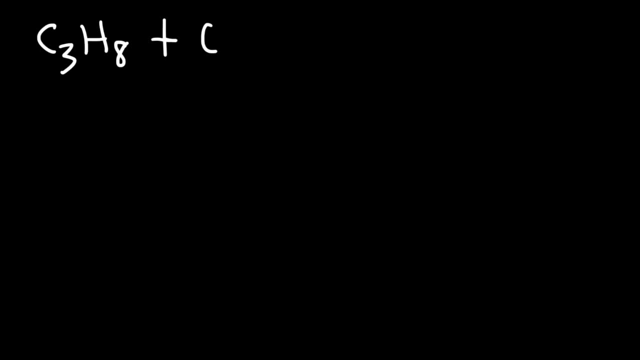 We're going to react propane- C3H8, with oxygen gas- O2, and it's going to produce carbon dioxide- CO2, plus water- H2O. So this time we have three elements that we need to balance in this chemical reaction. 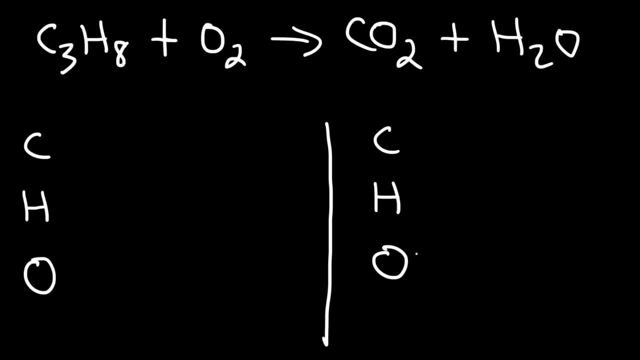 So this type of reaction is known as a combustion reaction. Whenever you have a chemical reaction, it's known as a combustion reaction. Whenever you have a chemical reaction, it's known as a combustion reaction. When you have a hydrocarbon like propane reacting with oxygen gas, it's always going. 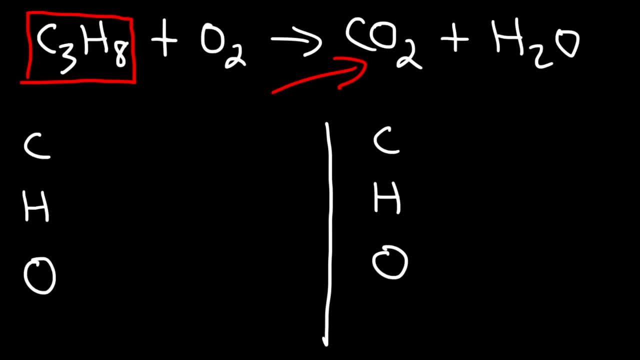 to produce products such as carbon dioxide and water. Now let's make a list of the number of atoms of each element that we have on both sides of the chemical equation. So on the left side or on the reactant side, we have three carbon atoms, eight hydrogen. 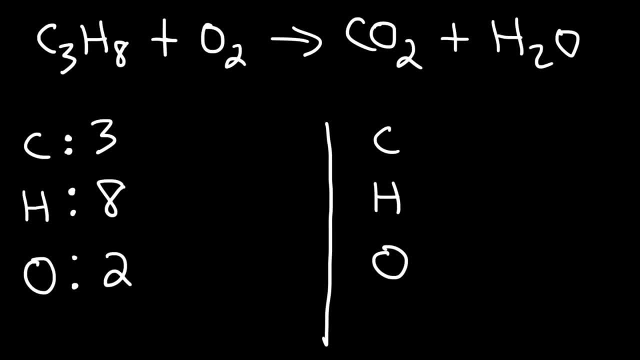 atoms and two oxygen atoms. On the right side we only have one carbon atom. now we have two hydrogen atoms and the number of oxygen atoms we need to perform addition because we have two in carbon dioxide but only one in H2O. 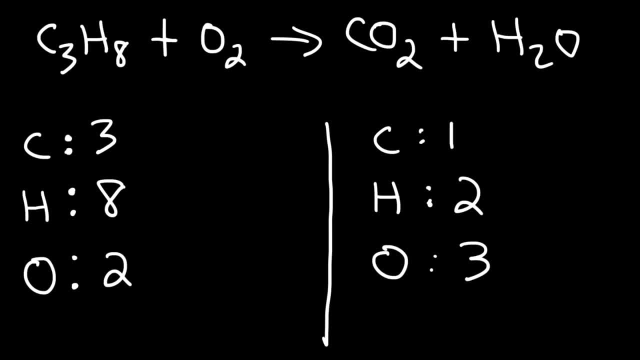 So two plus one will give us three. So now how do we go about balancing a combustion reaction? It turns out that for this type of chemical equation it's helpful to balance the carbon atoms first and then the hydrogen atoms second, and you want to save the oxygen atoms last. 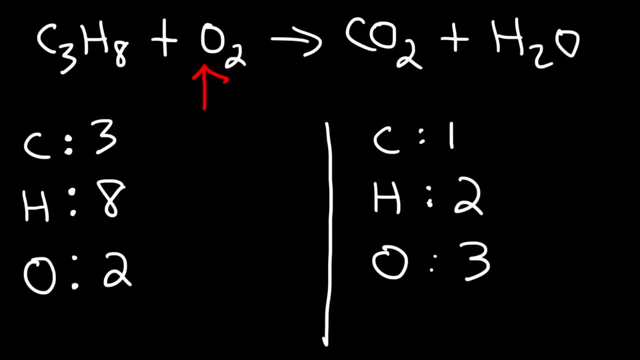 because you can easily adjust this number, since you have a pure element, since this substance only contains oxygen. So let's balance the carbon atoms. first, What we need to do is we have three on the left, one on the right, So we need to multiply one by three to get three. 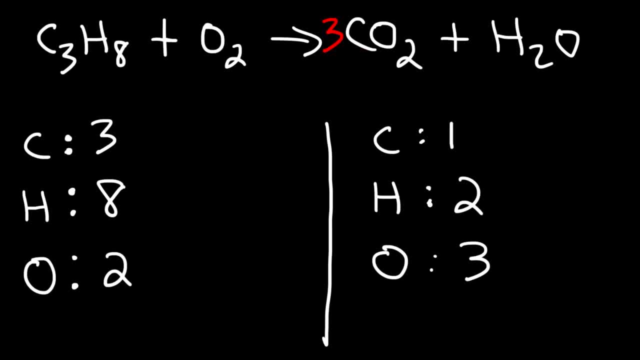 So let's put a three in front of CO2.. And so we're going to have three carbon atoms on the right side. Now this is going to change the number of oxygen atoms on the right side. So now this is three times two, which is six plus one. so now we have a total of seven. 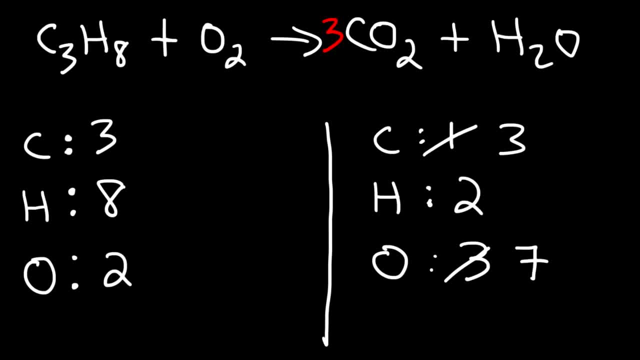 oxygen atoms on the right side. Now what about the hydrogen atoms? So we have eight on the left side, two on the right side. Eight divided by two is four. So this tells us that we need to put a four in front of H2O. 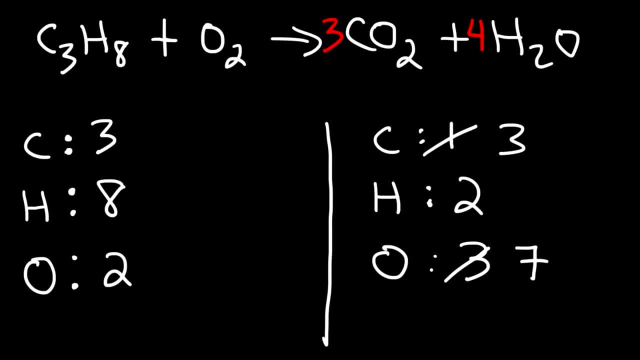 Four times two is eight. So now the number of hydrogen atoms on both sides of the equation are now the same. So the carbon atoms are equal and the hydrogen atoms are now equal. So the last thing we need to do is balance the oxygen atoms. 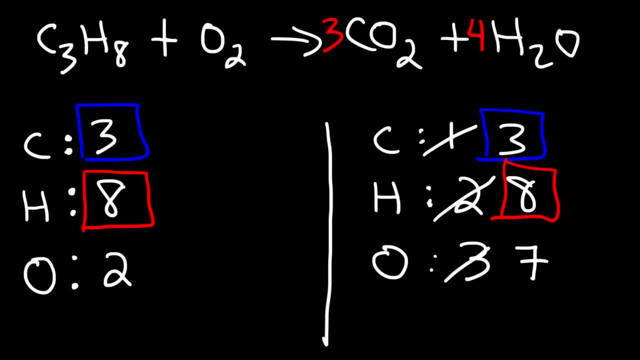 Now, by putting the four in front of H2O, we also change the oxygen atoms again, So we need to recalculate it. It's no longer seven Here. we have three times two, which is six, And four times one, which is four. 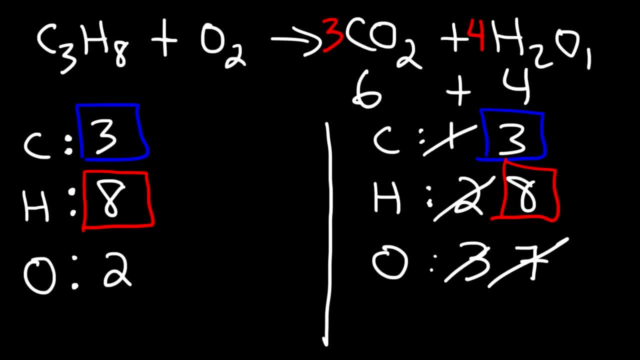 And so if we add six plus four that will give us ten. So we now have ten oxygen atoms on the right side. Now ten divided by two is five. So we need to put a five in front of O2, because five times two is ten. 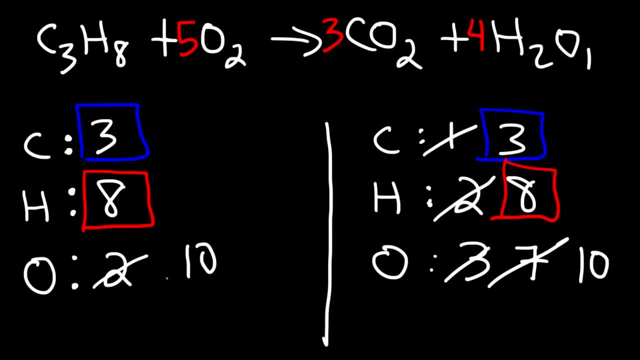 Now the number of oxygen atoms are the same, So we need to put a five in front of O2, because five times two is ten, And so at this point the chemical equation is balanced. So anytime you want to balance a combustion reaction like this one, I highly recommend. 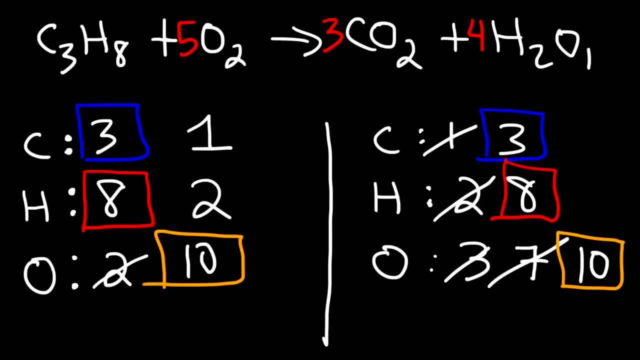 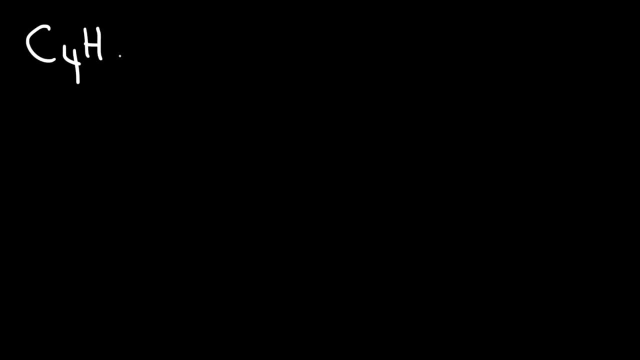 that you balance the carbon atoms first and then the hydrogen atoms second, and say, the oxygen atoms last. If you do it this way, your life will be a lot easier. Now let's try another example. So here we have butane. 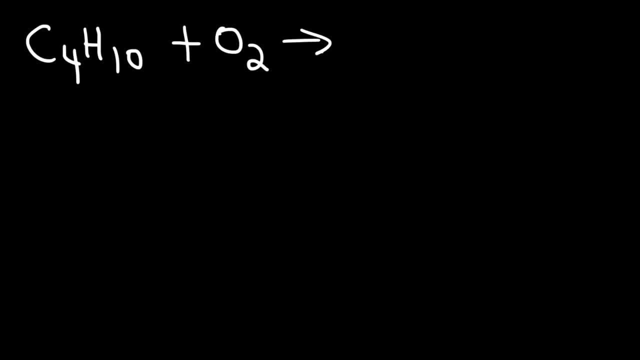 And here we have hydrogen And we're going to react it with oxygen gas to produce CO2 and water. So this is another combustion reaction, but it's a little bit different than the last one And you'll see. So go ahead and take a minute and try this example. 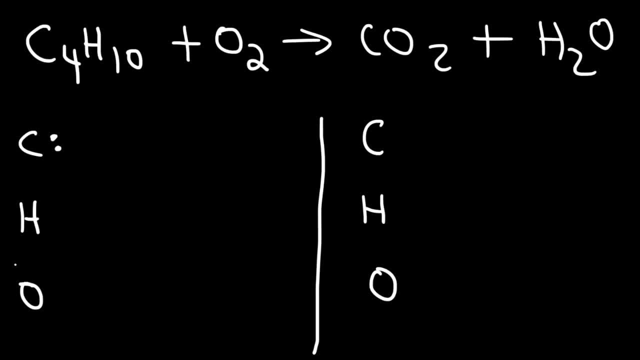 So on the left side we can clearly see that there are four carbon atoms, There are ten hydrogen atoms and two oxygen atoms. On the right side, we have one carbon atom, two hydrogen atoms and then two plus one. Don't forget about the invisible one. 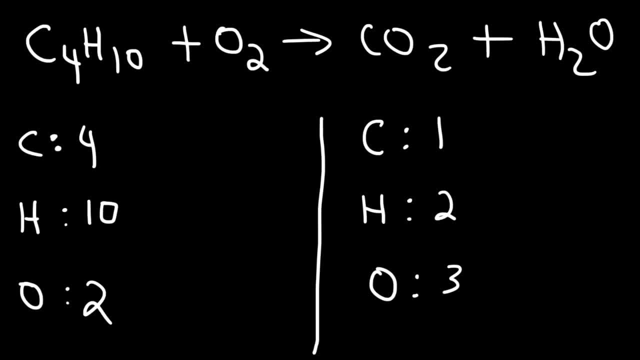 So we have three oxygen atoms. Now we're going to follow the same procedure. The first thing we're going to do is balance the number of carbon atoms, And so let's put a four in front of CO2.. So on the right side we're not going to have one anymore. 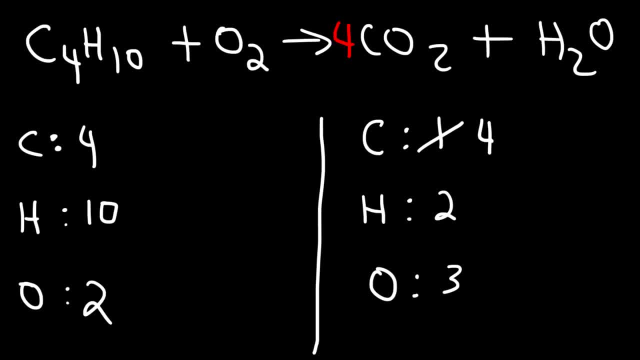 But we're going to have four carbon atoms. Next let's balance the number of hydrogen atoms. So ten divided by two is five. That tells us that we need to put a five in front of H2O. So now we have ten hydrogen atoms on both sides. 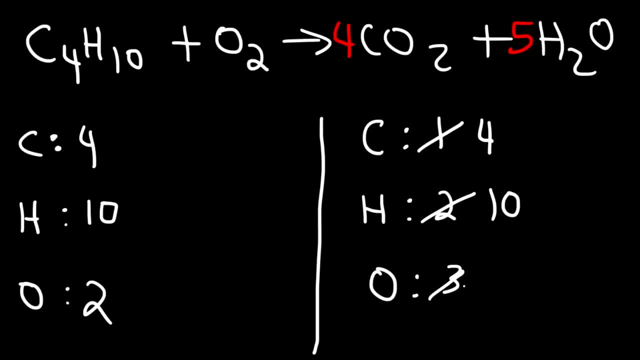 Now let's recalculate the number of oxygen atoms that we have. So four times two will give us eight, Okay. And then five times one is five. So eight plus five is thirteen. Now, thirteen divided by two is simply thirteen halves. So if we put thirteen over two in front of O2, the equation is balanced. 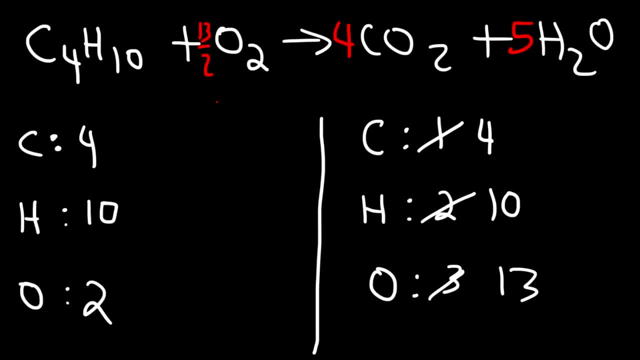 However, when you balance a typical chemical equation, You don't want fractional coefficients. Instead, you want whole numbers as your coefficients. And if you ever get to this point where you have thirteen over two a fraction, or six point five a decimal, what you need to do is multiply by a certain number. 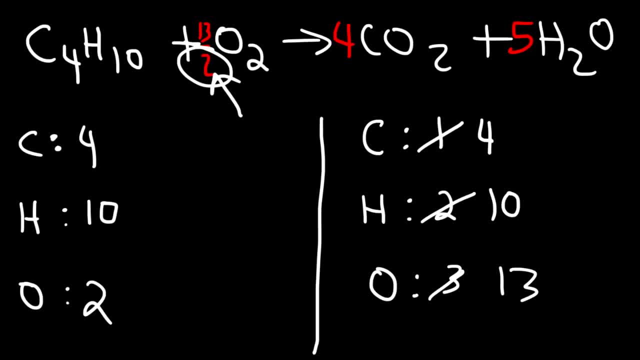 In this case, whatever the denominator is, you want to multiply it to get rid of that fraction. So what we're going to do is multiply everything by two. Okay, Thirteen over two times two, the twos will cancel, And so this is going to be thirteen now. 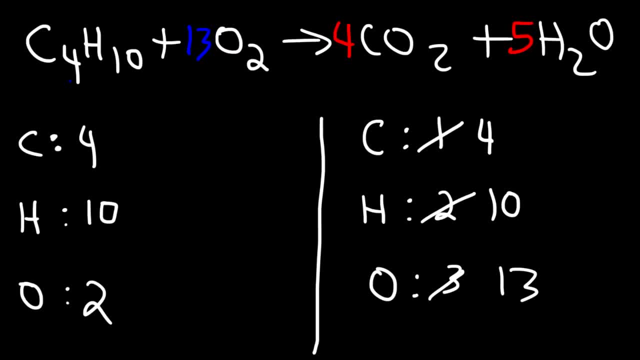 Here we had a one, but we're going to multiply that by two. So every coefficient that we see we're going to multiply by two. So four times two is eight And five times two is seven. Okay, And five times two is ten. 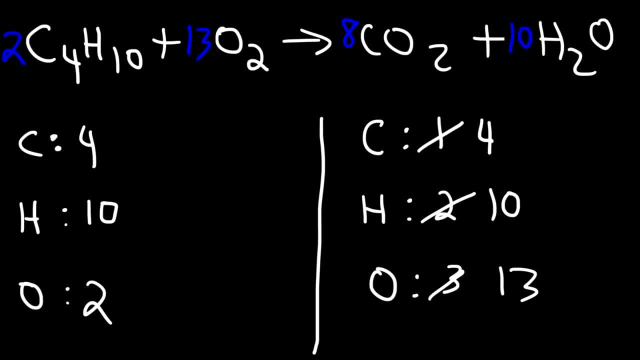 So now let's recalculate all the numbers that we have. So right now we have two times four or eight carbon atoms, And we have two times ten or twenty hydrogen atoms on the left side, And for oxygen it's thirteen times two, which is twenty-six. 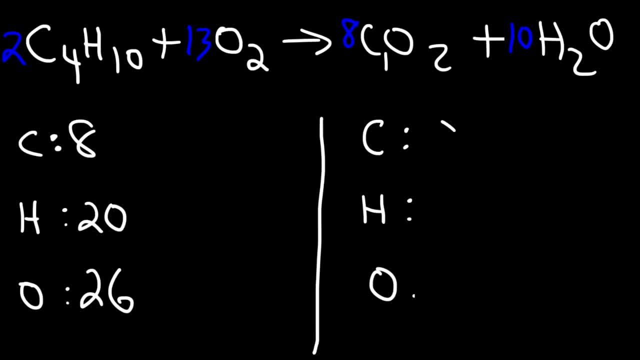 Now, on the right side, we have eight times one or eight carbon atoms, And for hydrogen it's ten times two, which is twenty, And in the case of oxygen it's eight times two, which is sixteen plus ten times one. 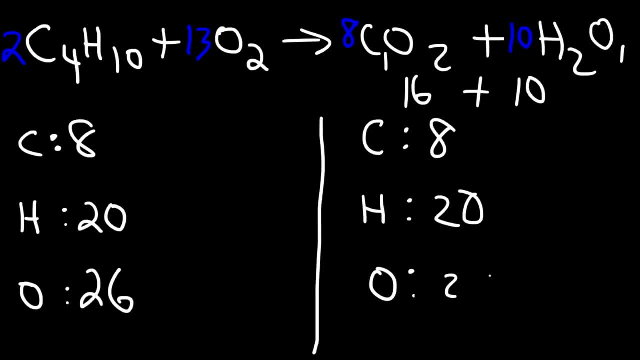 which is ten. Sixteen plus ten is twenty, It's twenty-six. So we can clearly see that the number of carbon atoms are the same, The number of hydrogen atoms are equal on both sides, as well as the number of oxygen atoms. 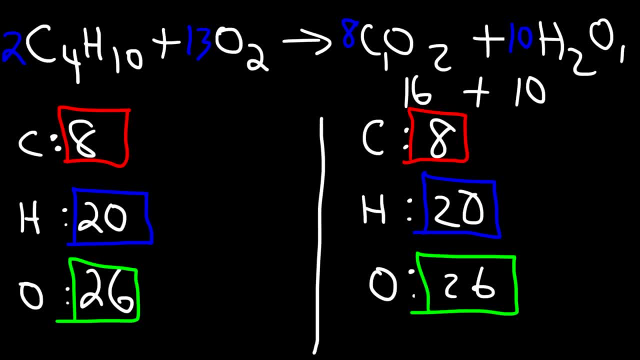 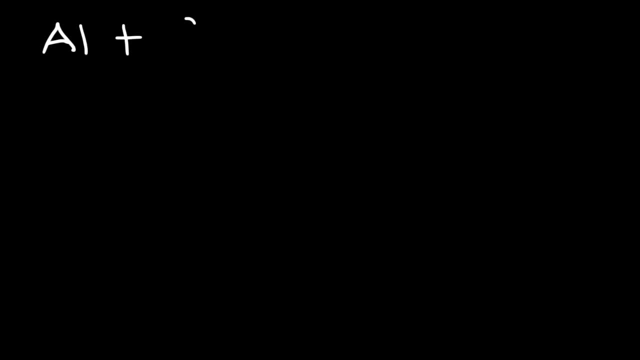 And so that is how you can balance a combustion reaction. Now let's talk about how to balance a single replacement reaction. So here we have aluminum. We have aluminum reacting with copper chloride and it's going to produce aluminum chloride plus copper. Take a minute and try this problem. 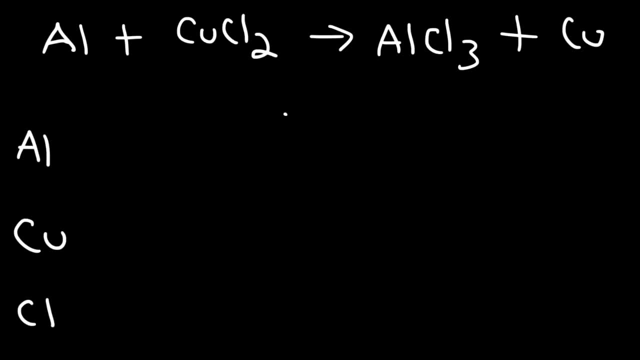 So we have aluminum, copper and chlorine. So on the left side we can see we have one aluminum atom and we have one copper atom, but we have two chlorine atoms. On the right side we have two chlorine atoms. On the right side we have two chlorine atoms. 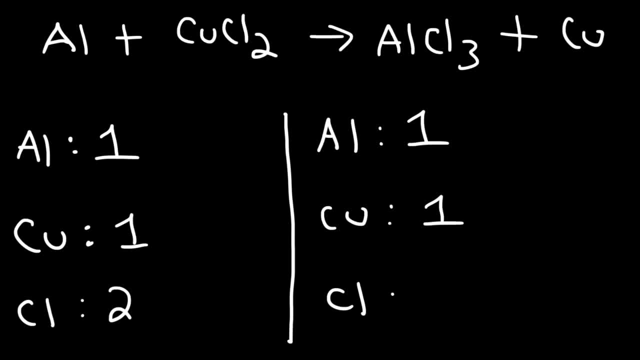 We have one aluminum atom, one copper atom and three chlorine atoms, So this problem doesn't look too bad. The only thing that is different at the moment is the number of chlorine atoms. So how do we make them equal? Well, we need to find the LCM, the least common multiple of two and three. 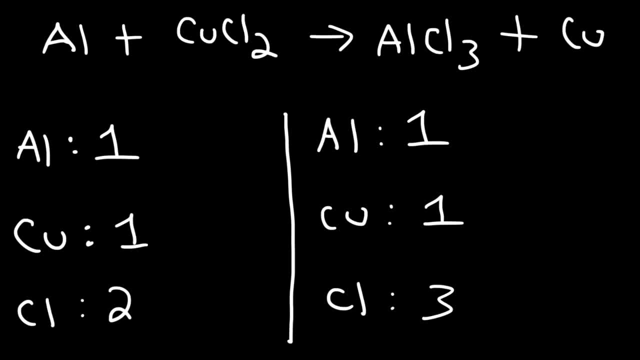 Two times three is six, And so what we want to do is we want to get six chlorine atoms on both sides of the equation. So we're going to do that. To get six on the left, we need to put a three in front of CuCl2, because three times two, 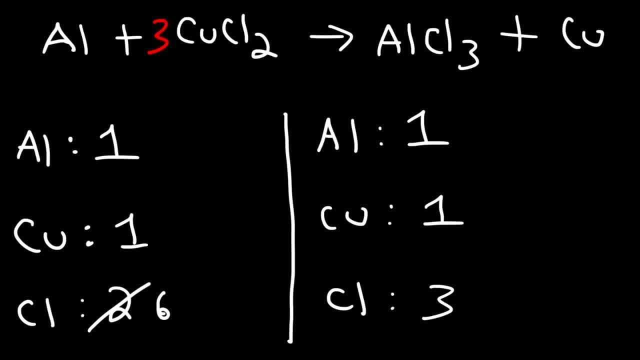 will give us six. Now, on the right side, we need to put a two in front of AlCl3,, because two times three will also give us six. Now the number of chlorine atoms are the same, But by adding these numbers we're going to get a two. 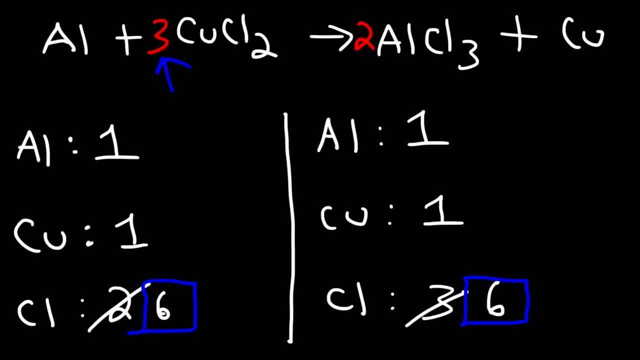 We need to put a three in front of CuCl2, because three times two will give us six. the number of copper atoms and aluminum atoms changes. So on the left side we no longer have one copper atom, We have three copper atoms. 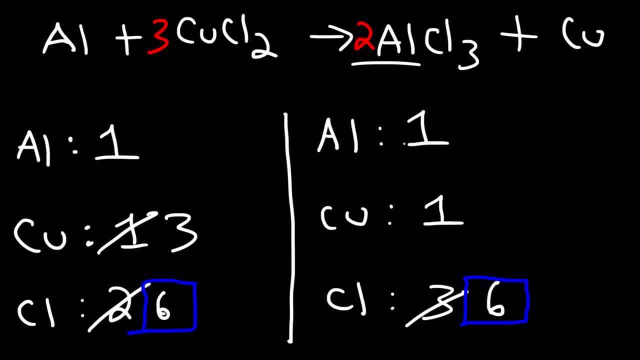 On the right side. we no longer have two aluminum atoms. I mean we no longer have one, but we have two aluminum atoms. Now to balance the number of aluminum atoms, we need to put a 2 on the left side in front of Al. 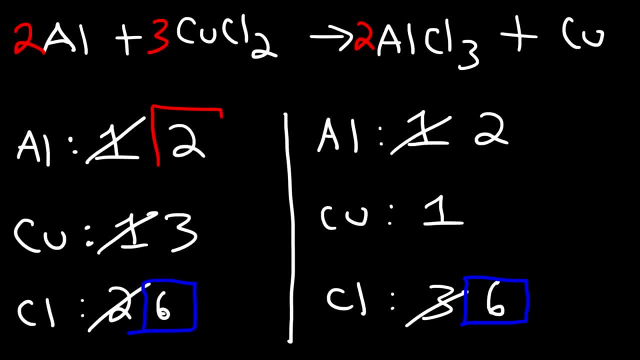 So this changes to 2.. And so now these are the same, And in the case of copper we need to put a 3 in front of Cu, so that there's three copper atoms on the right side. So now the number of aluminum atoms, copper atoms and chlorine atoms. 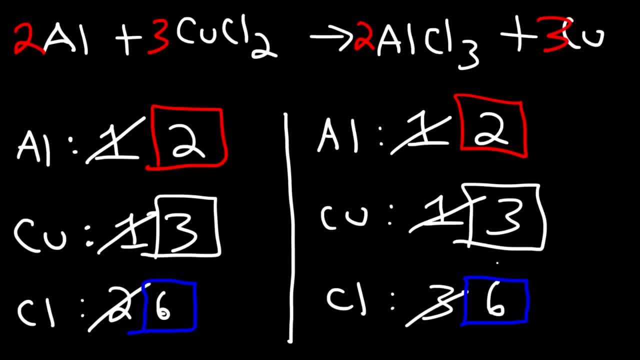 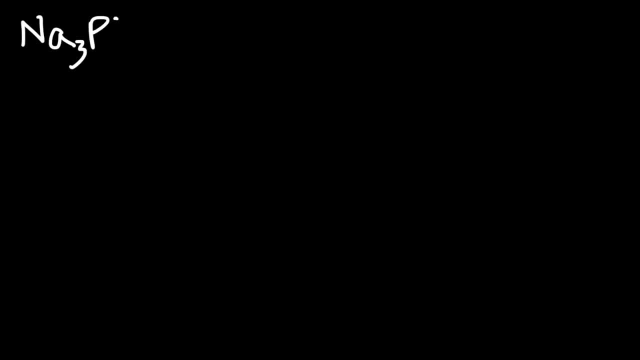 are the same on both sides, And that's it. That's all you've got to do in this example. Now here is a harder example. So this is called a double replacement reaction. We're going to make sodium phosphate with calcium chloride. 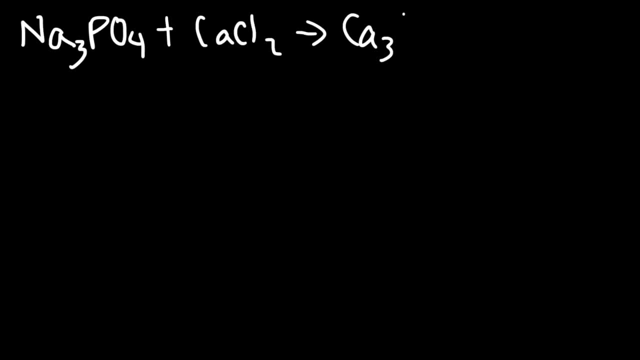 And we're going to get calcium phosphate, Ca3PO42, plus sodium chloride. Now for a double replacement reaction like this with those that include polyatomic ions, in this case phosphate. I don't recommend that you balance every element individually. 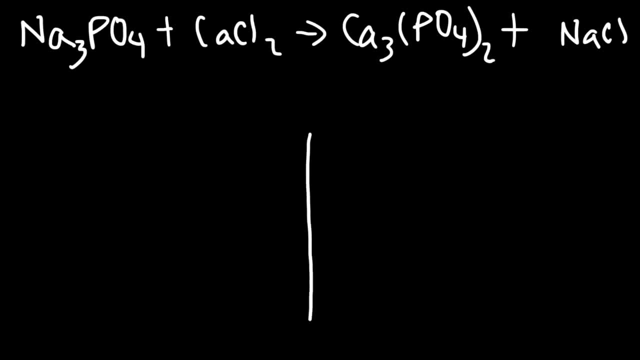 Instead, you should balance individual ions And it helps to know the polyatomic ions. So you need to balance the sodium ions separately, the calcium ions, the chloride ions and the phosphate ions. You need to see PO4 as one unit for this particular reaction. 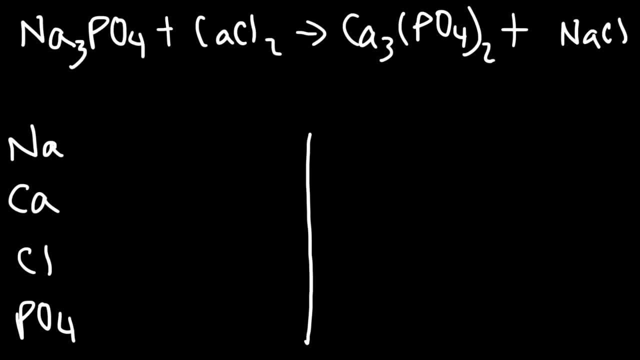 If you try to separate the phosphorus and the sodium, you're going to get a 2. If you try to separate the phosphorus and the oxygen atoms, it could be a challenge, particularly if there's another polyatomic ion, Let's say, instead of sodium chloride. 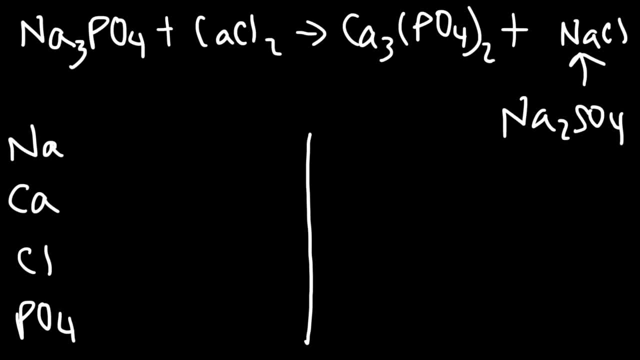 we had sodium sulfate. Trying to balance the elements separately in that case will be a disaster. So I highly recommend that you balance the phosphate unit PO4, rather than separating the elements. For this particular example, it's going to be very useful that you do that. 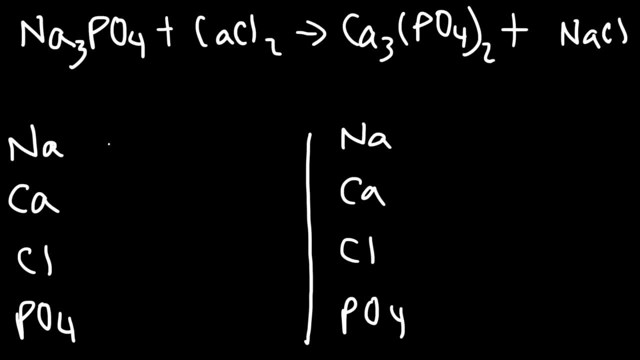 So right now, on the left side, we have 3 sodium ions, 2 calcium ions- I mean not 2, but 1,- 2 chlorine particles and 1 phosphate ion. On the right side, we have 1 sodium ion. 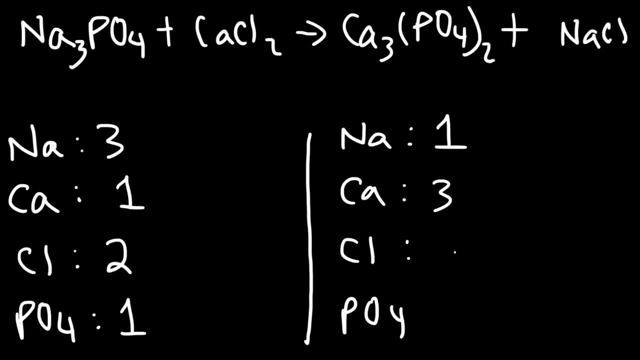 3 calcium ions, 1 chloride ion, and here we have. we have 2 phosphate ions, based on the subscript. that's here. So which one should we balance first? Typically, I like to start with the polyatomic ions, the ones with the highest charge. 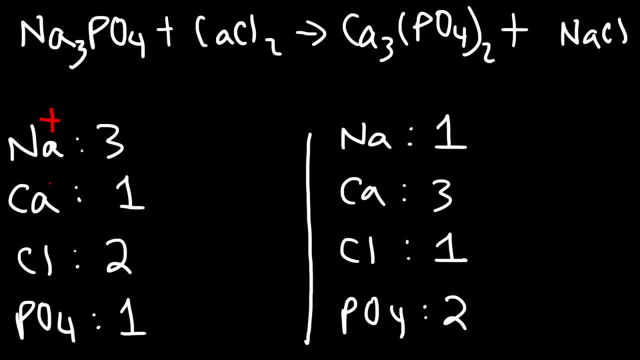 Sodium has a plus 1 charge. It's found in group 1 of the periodic table. Calcium has a positive 2 charge, or sometimes written as a 2 plus charge. It's found in group 2 of the periodic table. 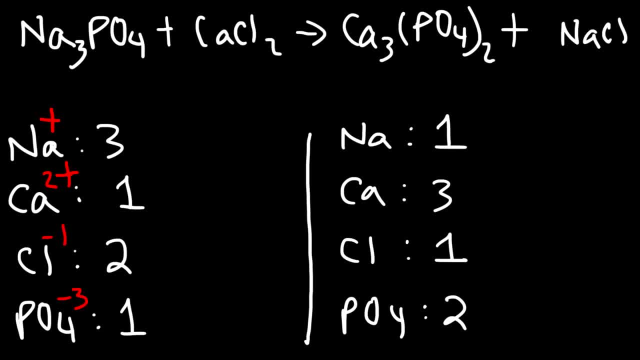 Chlorine has a minus 1 charge and phosphate has a negative 3 charge. If you haven't learned this, don't worry about it. You can still balance it without this information. But if you know it, it's better to balance the charges. 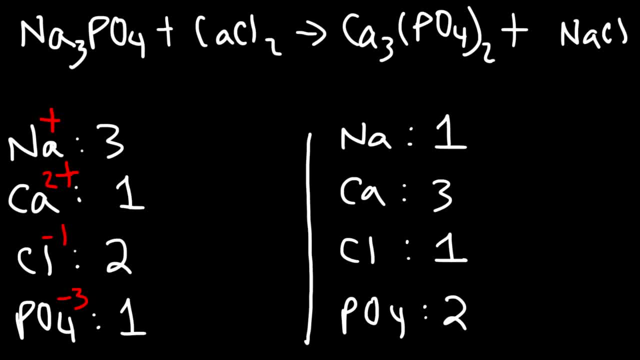 the ions with the highest charge, In this case the phosphate ion, And my experience has been easier that way. So what I'm going to do is put a 2 in front of sodium phosphate so that the phosphate ions are balanced. So we have 2 on both sides. 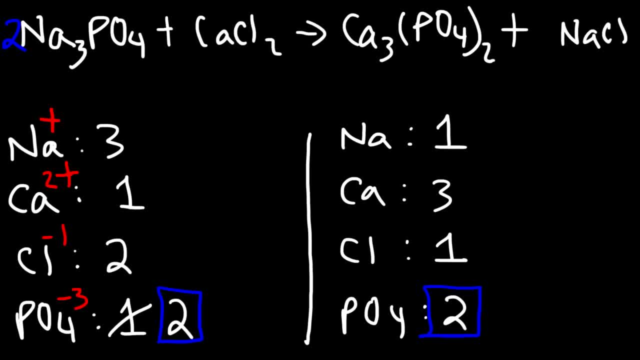 Now I won't have to change that anymore, You'll see. Next, let's balance the sodium ions. On the left side, we have 2 times 3, which is 6.. So this changes. Now we have 1 on the right side. 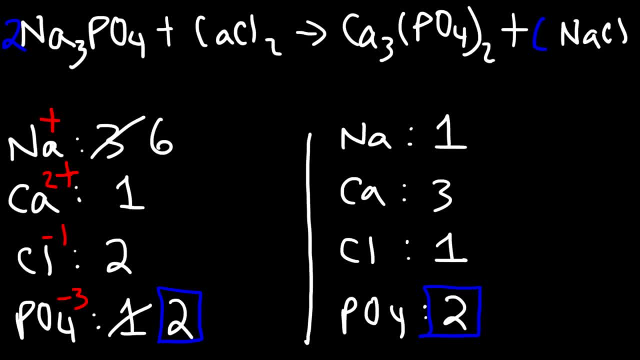 so we've got to multiply that by 6.. So let's put a 6 in front of NaCl, So now we have 6 sodium ions on both sides. Now by putting the 6, we change the number of chloride ions.